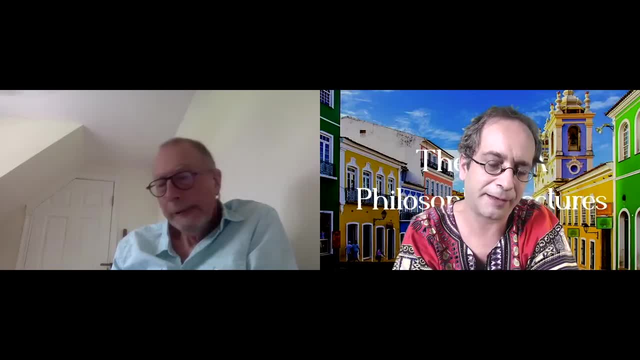 And this, well, an important part of his proof is the fact that these sentences about the language of arithmetics can actually be mapped onto sentences of arithmetics itself, And, aside from that, they can actually refer to themselves, and these are two aspects that surely Russell had in mind. 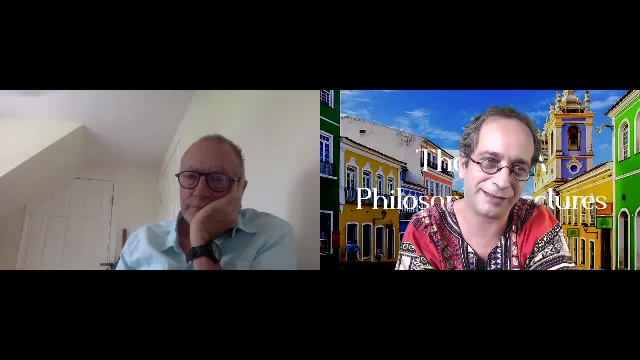 Especially the possibility to be self-referential, because he would have immediately thought that something was wrong. I suppose if he had suspected that this was possible, Could you tell us how this was possible? How could you go about proving that sentences about arithmetics can be systematically mapped onto sentences of arithmetics? 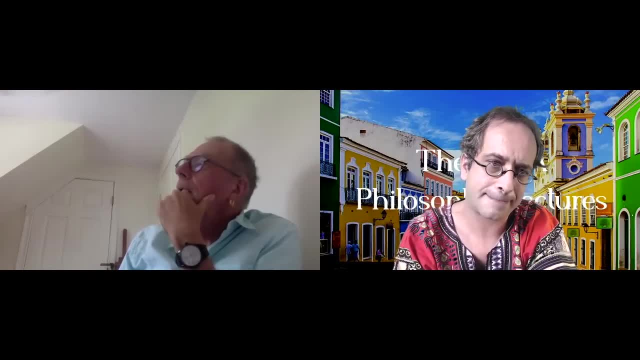 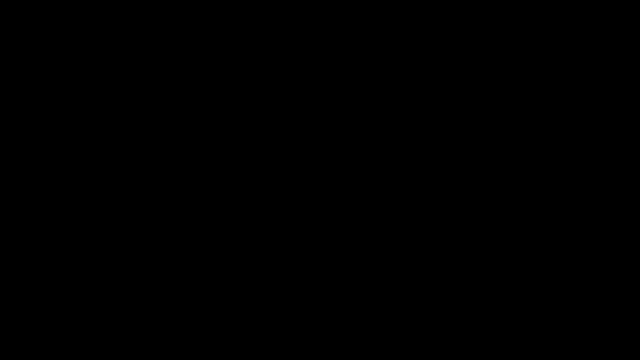 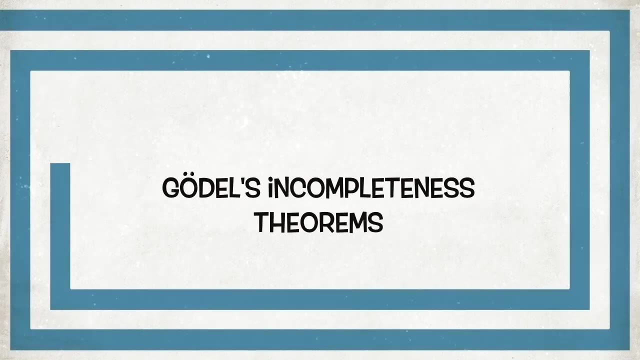 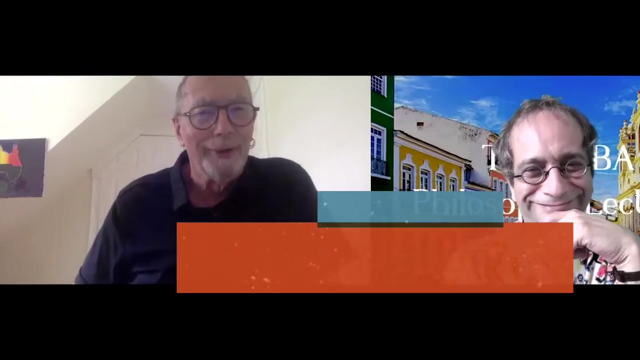 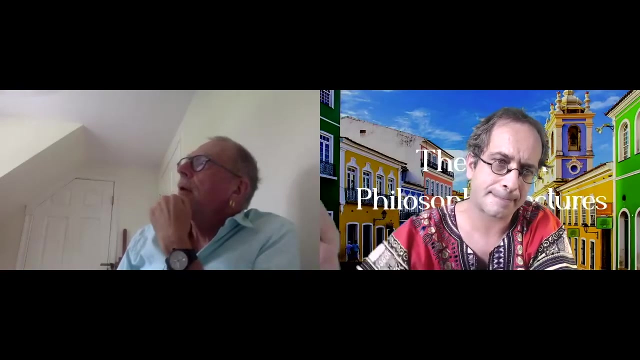 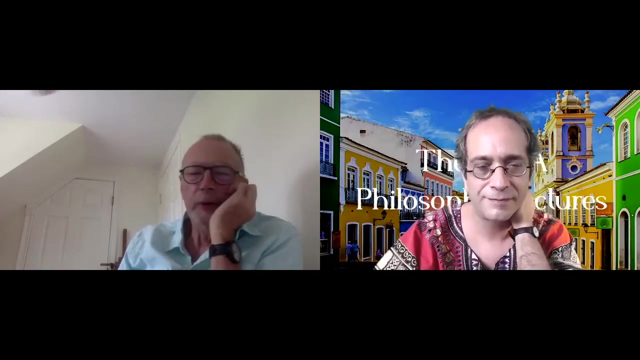 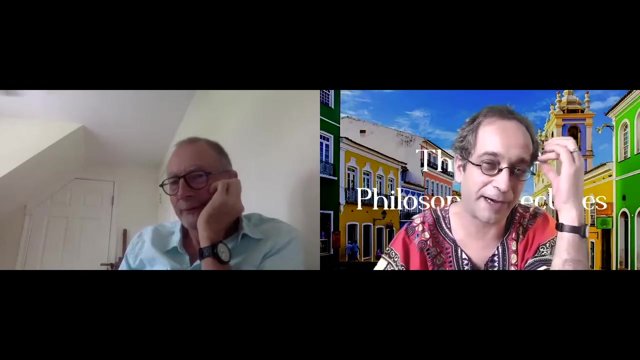 Yeah, Okay, look what Russell's reaction to Gerdel's theorem was. I'm not sure. I'm sure he must have talked about it somewhere, but by this time he was losing interest in mathematics anyway, I'm not sure. I was reading yesterday, but I couldn't find the reference that he said something. oh, right then should we believe that 4 is equal to 1.5, or something like that? 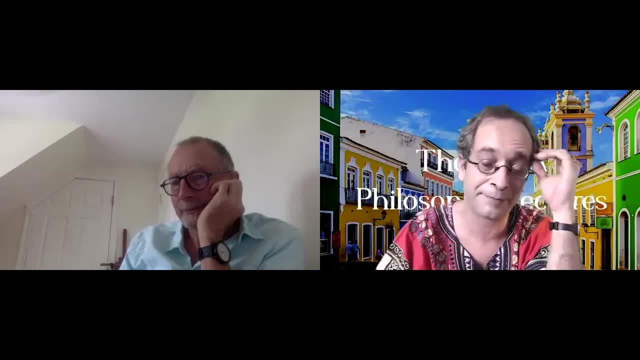 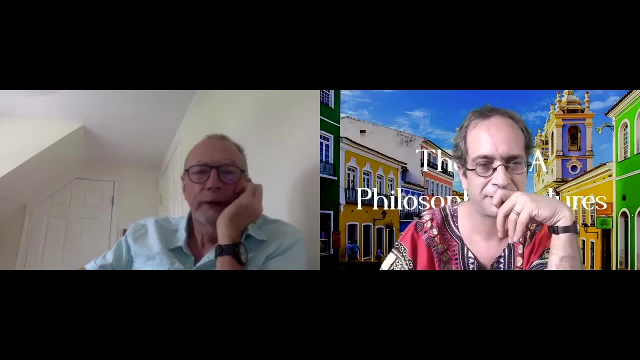 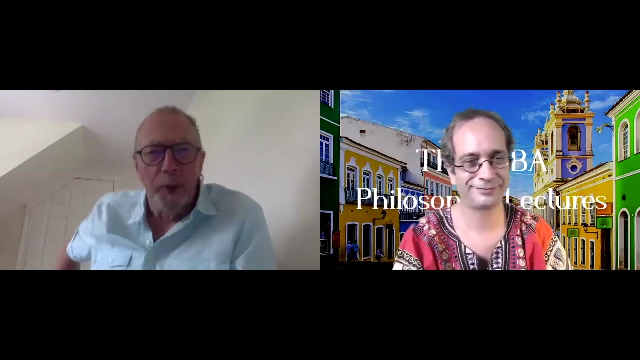 But I'm not sure whether I couldn't find the reference. so I'm not sure. Okay, I'm not sure whether this is true. Yeah, well, look, I'm sure that some of the Russell aficionados out there in the greater world will know what Russell made of it, and probably you know. if you have a blog page, they'll write and they'll tell you, but I can't remember. 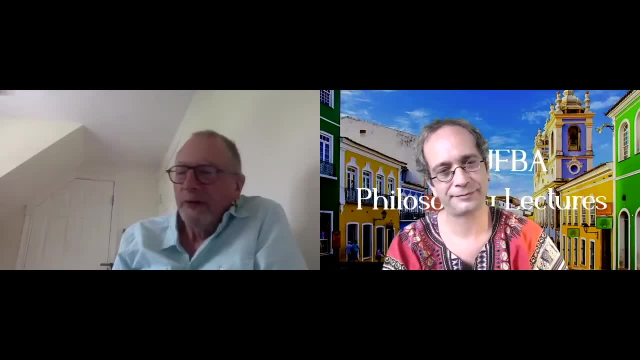 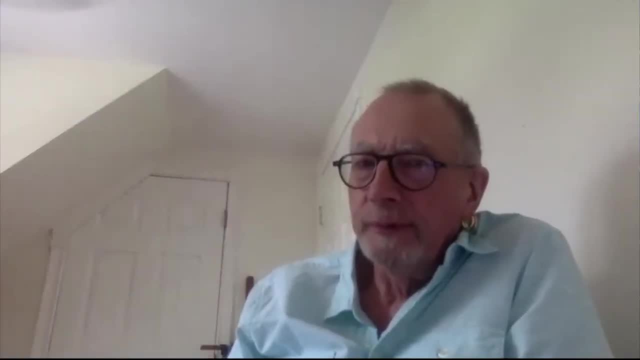 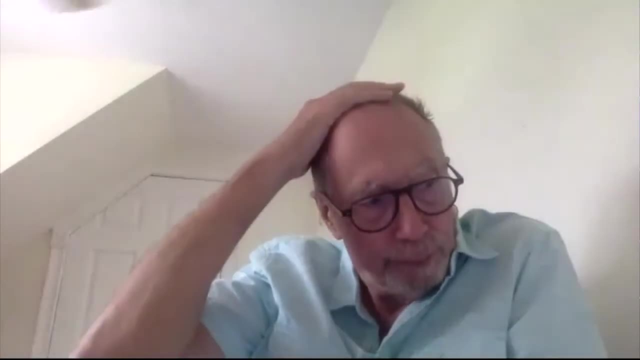 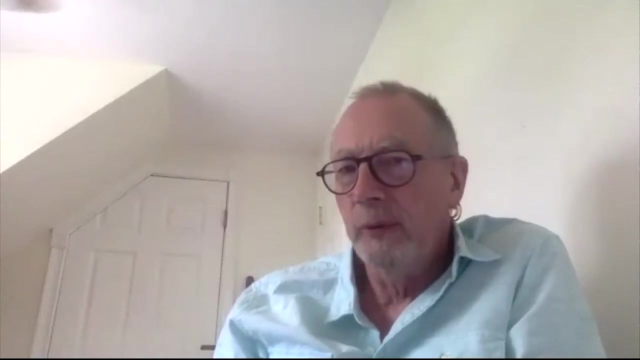 Okay, so set Russell aside. Look, there are a number of different proofs of Gerdel's theorem. He came up with the first, but we know several more now. Some of these appeared when recursion theory developed in a more systematic form, 10, 15 years later, in the work of people like Turing and so on. 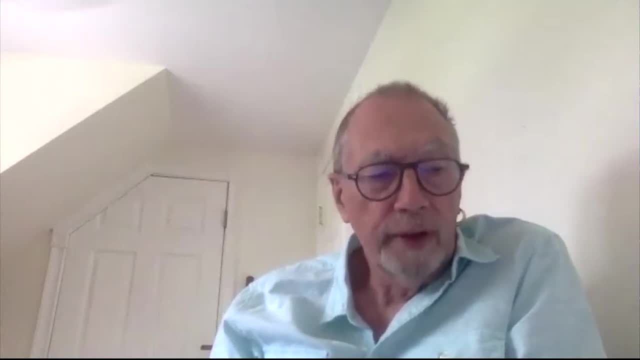 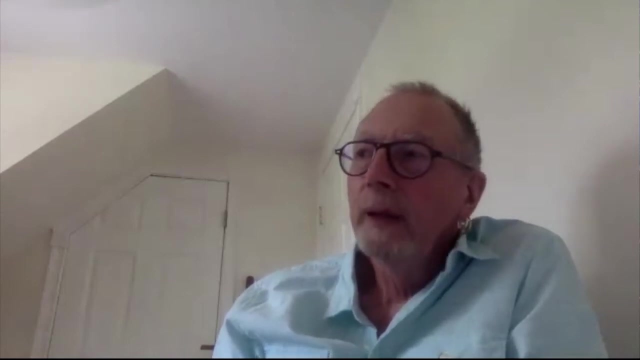 But all the proofs that I know do depend on the fact that you can code things as numbers. Okay, Okay. So these might be computer programs or these might be proofs, and so on. So this coding technique is central to all the proofs that I know, and it was a technique that was developed by Gerdel. 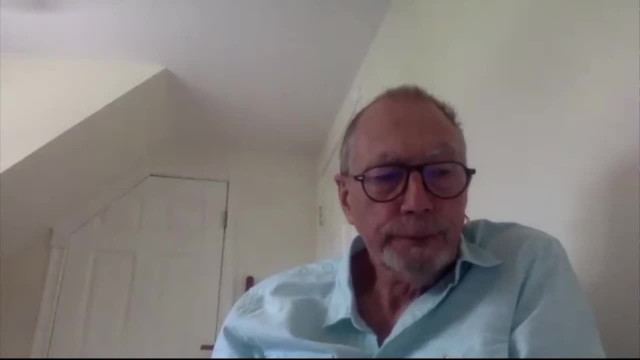 So let's come back to that in a second. There is a clear analogy between Gerdel's proof of incompleteness and the liar paradox. So we've talked about the liar paradox before. So the form of this sentence is not true. If it's true, it's not true. 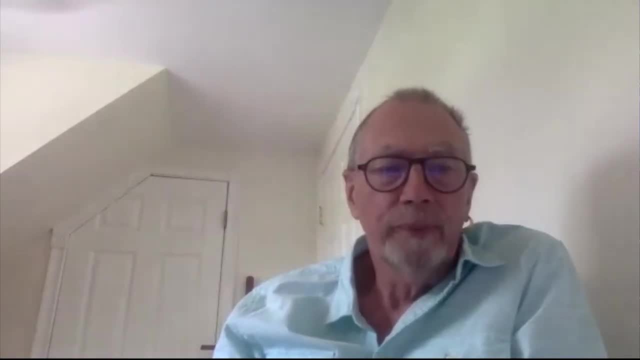 If it's not true, it's true. So you have a problem. And in fact that was used. That argument was used by Tarski In the late 20s, early 30s to prove that the concept of truth for an arithmetic sentence is not definable arithmetic. 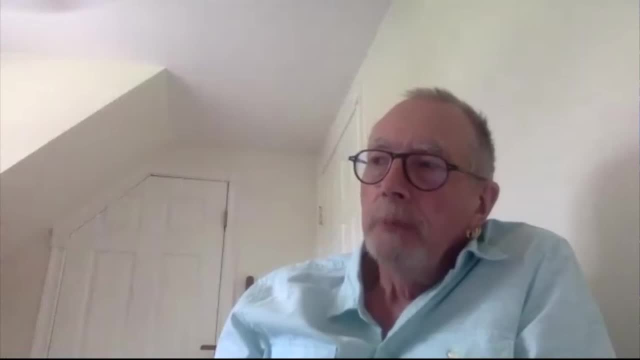 It's actually used the liar paradox, right, But what Gerdel does is not use the liar paradox, but a paradox of provability which is very, very similar. I mean, I've called it the provability paradox or Gerdel's paradox. As you said, it concerns the sentence. It's not the case that this sentence is provable. OK, so suppose it's provable. Well then it's true. So it's not provable. So it can't be provable by reductio or whatever. 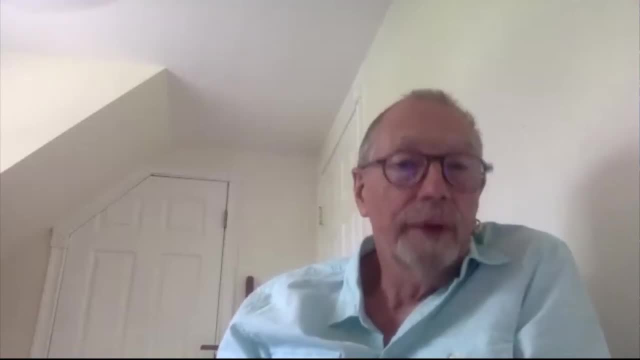 And we've just proved this, So it is provable. OK, that's Gerdel's paradox, And clearly his proof of incompleteness applies. this in some sense Was he trying to prove the inconsistency of arithmetic and the incomplete result fell out. 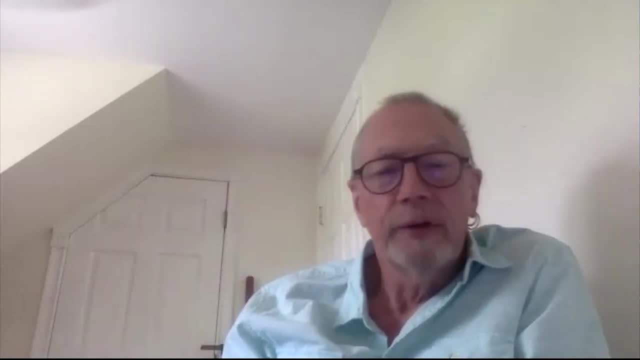 I don't know. I don't know that anyone has commented on this, But this argument is certainly a driving bit of the argument. It turns out that, given that you can represent this kind of argument about provability in arithmetic, you might think: well, hey, why doesn't it show that arithmetic is inconsistent? 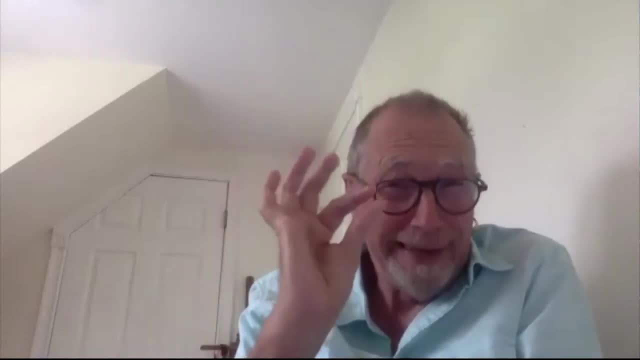 And the answer is that it sort of fails by a head's breadth. We can go into that, if you like. Why? Because there's just one very crucial small step at which you can't push the argument through. Yeah, let's get into that. 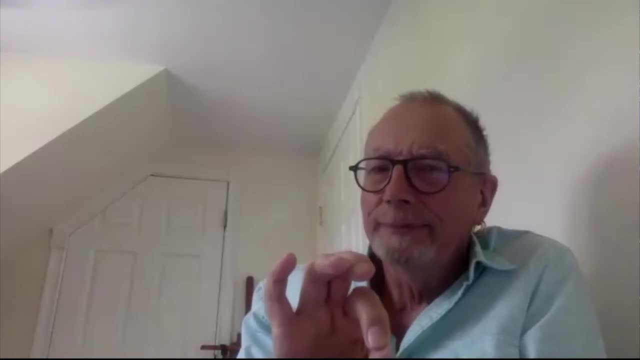 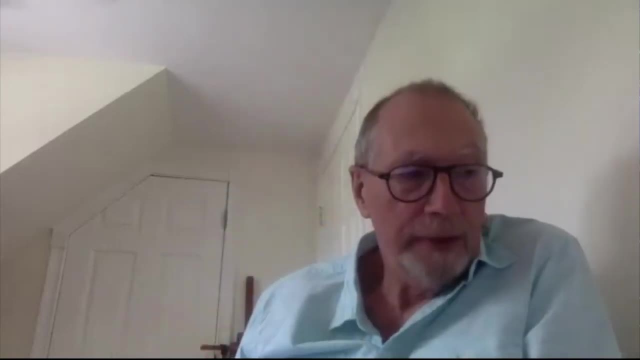 You want to talk about that now? We haven't talked about that. Oh, whenever you think it's most Well, we can deal with that now. So if you take your mind back to this provability argument- Cooberty-Parrock's argument I gave you it said: OK, so the sentence is, this sentence is not provable. 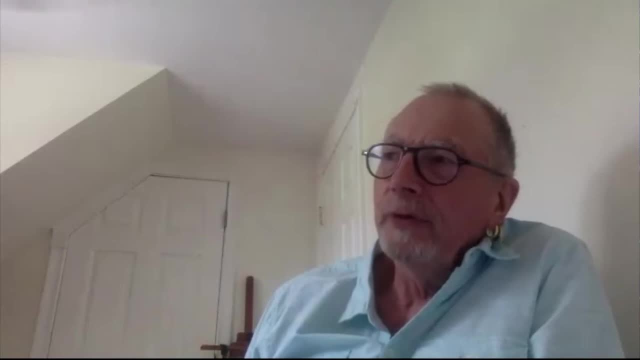 Suppose it's provable, Then it's true. So it's not provable. OK, In fact, you don't need to invoke truth here. All you need to invoke is that if you can prove A, then A, You don't have to mention truth. 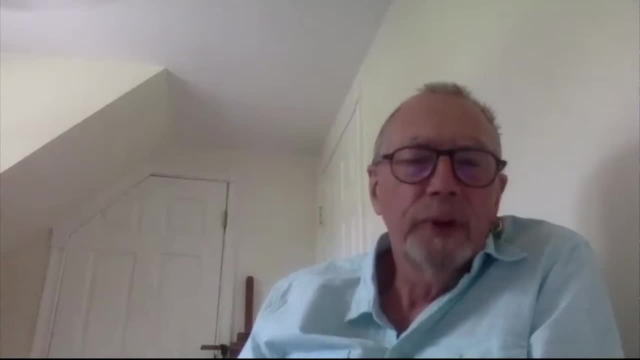 So it appeals to this principle that if A is provable, then A, And you cannot establish this. You cannot establish this in axiomatization to arithmetic, at least if they're consistent, because then you can push through the argument. So there are instances of this principle which cannot be proved in arithmetic. 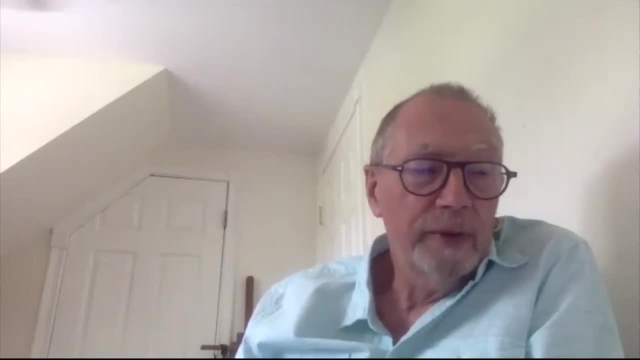 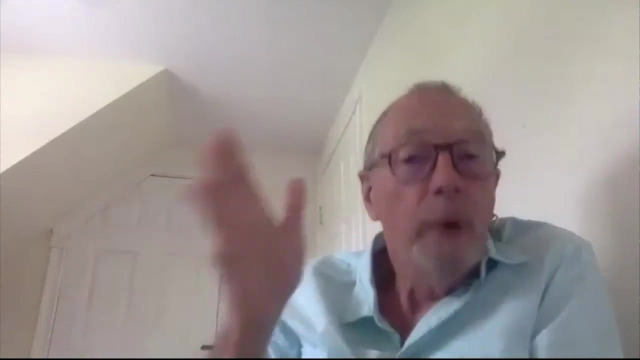 In fact, there was a result established some years later- I'm not sure of the exact date- by Loeb, who showed this. Suppose you can prove something of the form. If A is provable, then A, then A must already be provable. 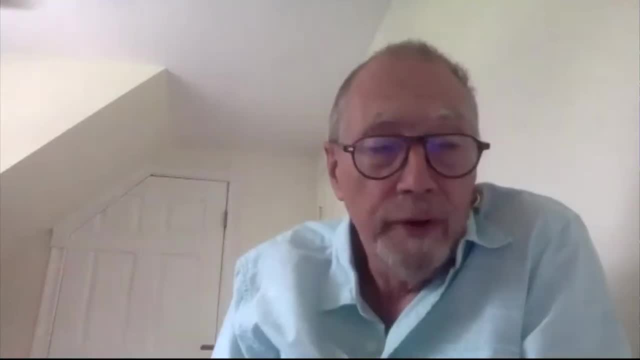 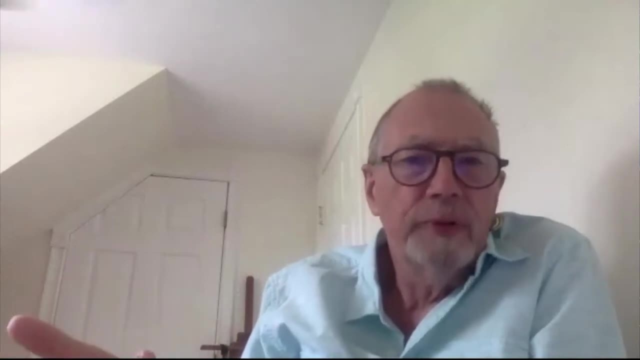 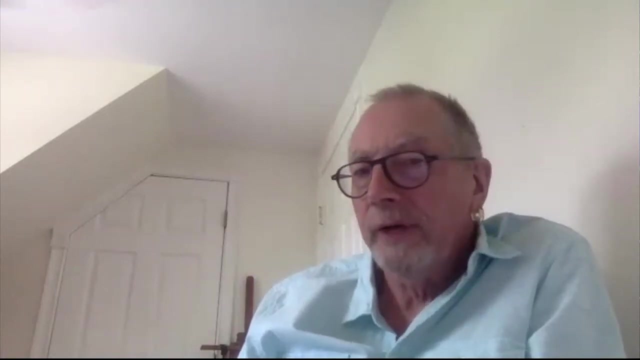 Because it's supposed to hold for everything. Intuitively it's true for everything, But given a consistent arithmetic, you can only prove the instances for those A that are already provable. So you know, it's another kind of way of getting at Gödel's incompleteness theorem. 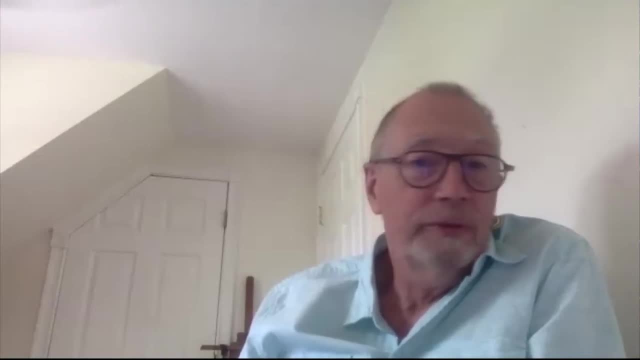 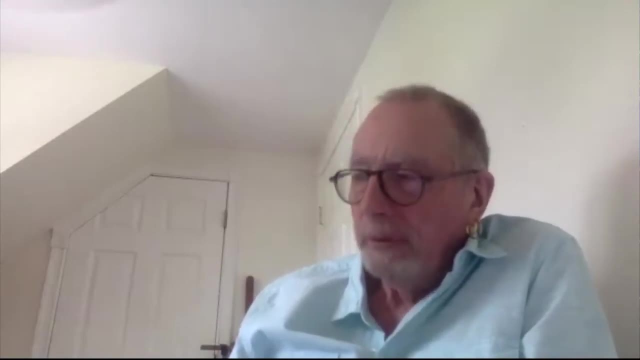 Because here are some things which you can't make. There are some things which are absolutely true in the standard model but which you can't prove. So you cannot push through the Gödel paradox argument on pain of inconsistency. All right, So do you want to continue with that or do you want to go back to provability? 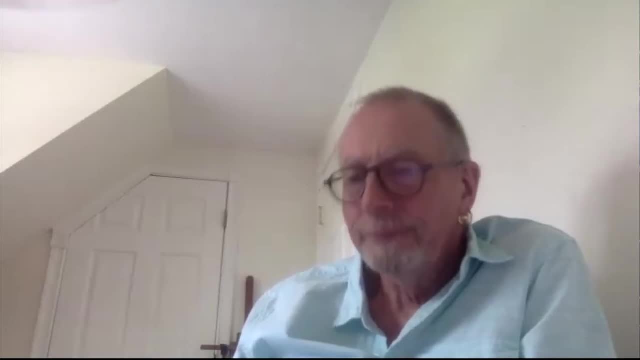 Well, let's go back to provability. So this is all on the assumption that you can express things like the apparently a paradoxical sentence as a purely arithmetical sentence. In other words, you've got to phrase it in such a way that you're only talking about numbers. 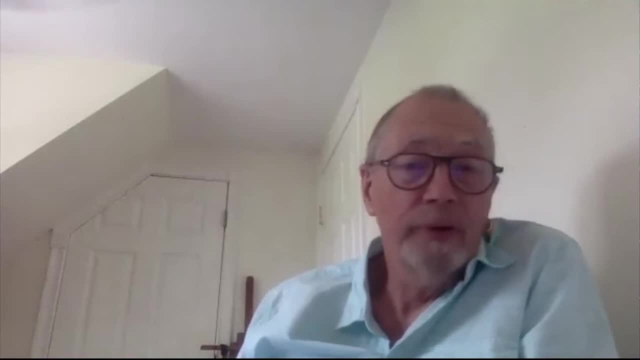 Because provability isn't about numbers, It's about axiom systems. But one of the clever things about Gödel's proof is that he showed how you could express facts about provability and so on simply in terms of numbers, And you do this by coding. 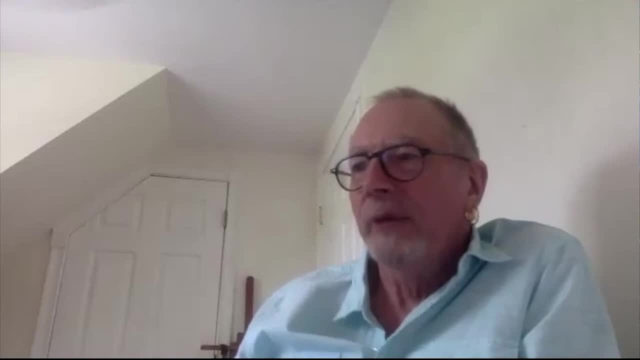 And coding is kind of easy when you, you know, sometimes kids play this game And you do this by coding, And coding is kind of easy when you, you know, sometimes kids play this game. But I'm going to write you a coded message. 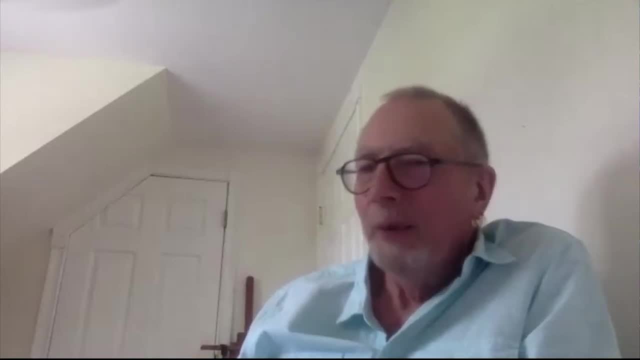 I'm going to write you a coded message, Right? But I don't want people to know about it, So this is what I'm going to do. I'm going to assign A- the number 1,, B- the number 2,, C- the number 3, and so on. 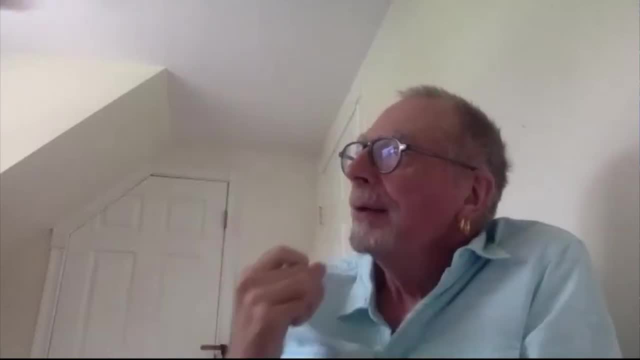 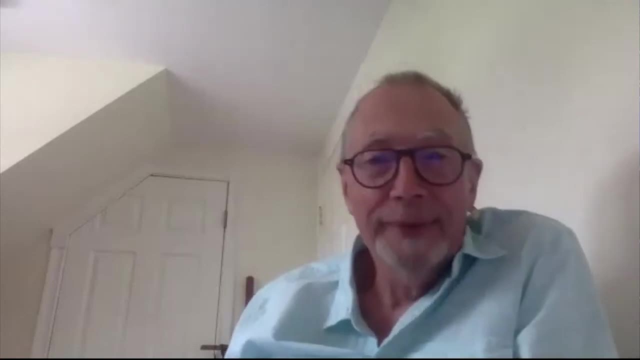 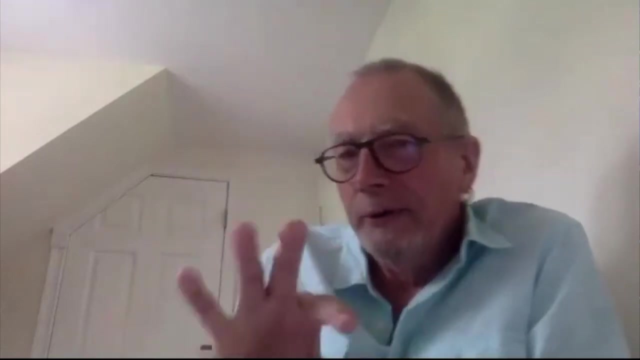 And now I'm going to write my message to you as a sequence of numbers. So instead of I don't know, I can't do this in my head, you write one, two, three, okay, and you know the code and you can decode. so if you know the codes, 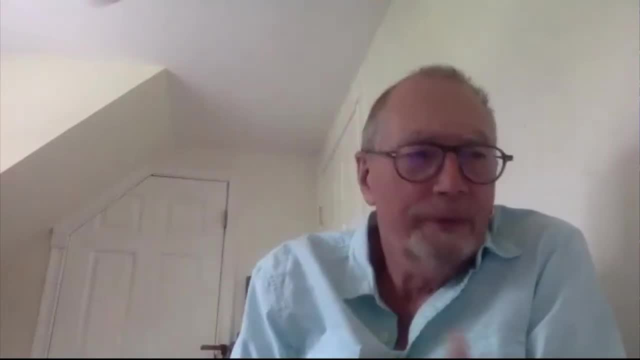 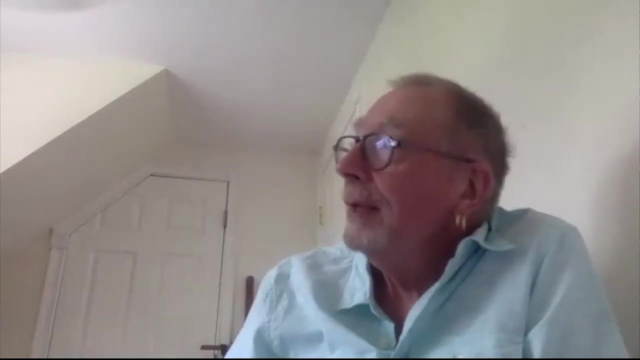 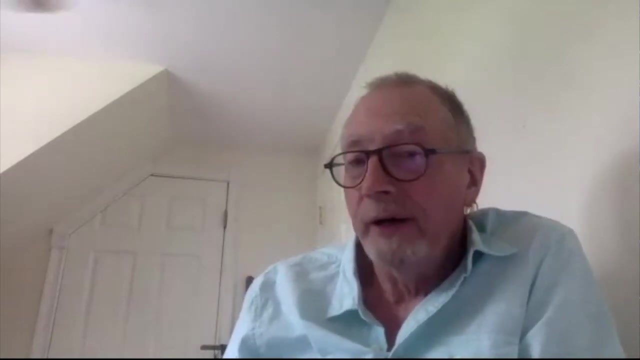 and you know how to decode, then you can express the centers of english in terms of numbers, a sequence of numbers. well, actually, because it's a finite sequence of numbers and, as is well known, you can code up any finite sequence of numbers itself as a number, so you can reduce this just. 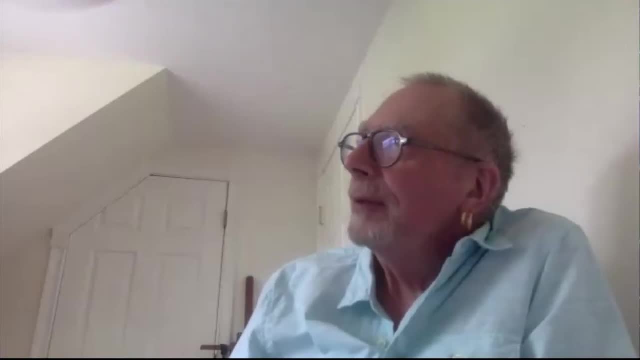 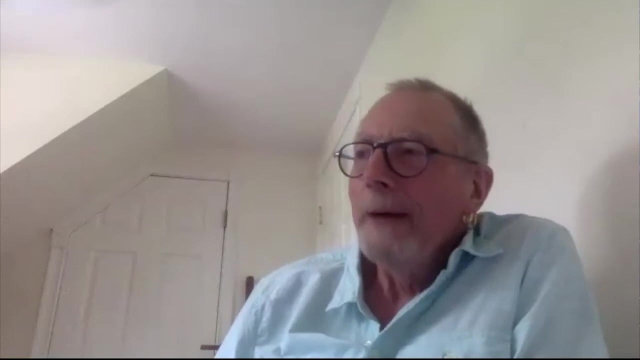 to a single number. so i mean i might um send you a code saying: uh hey, miliano, um, six million four thousand nine hundred and seventy two- huh, how about that? and you get your piece of paper out, you do the decoding right and you know what i said, all right. so what girdle showed was this: 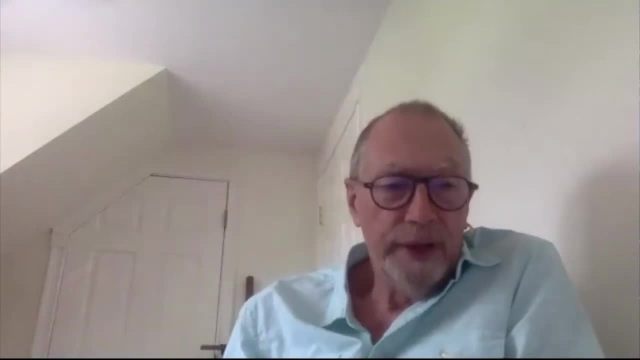 with this sort of notion of coding was that you can express facts about um sequence sentences. you can express facts about um sequence sentences and you can express facts about um. sentences are codes, have codes, sequences of sentences have codes and therefore proofs have codes. so, um, instead of talking about a proof, you can talk about this code number. 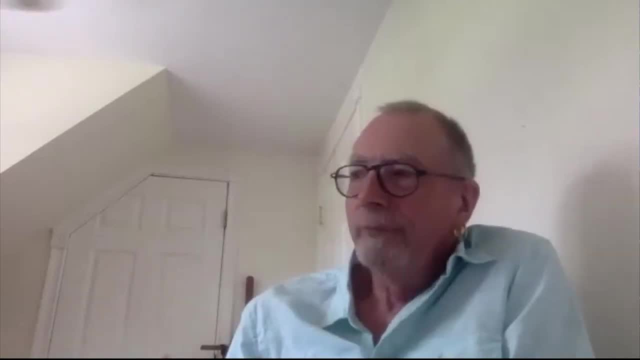 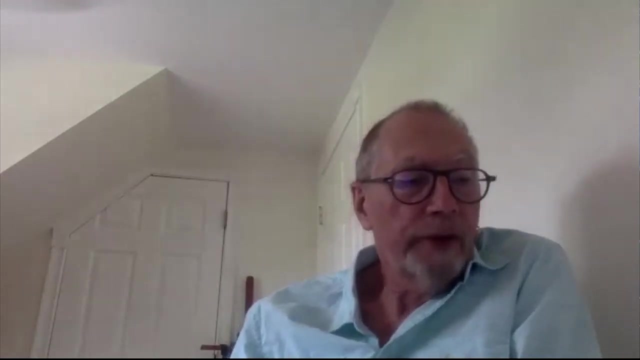 um, and because there's a kind of um, a two-way map between the code and what it codes, then anything you can express about proofs you can express by a number. so this is how you can um, express things about provability simply as a fact about numbers, okay, um. 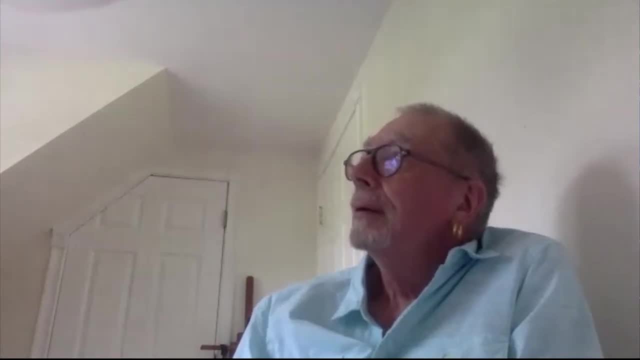 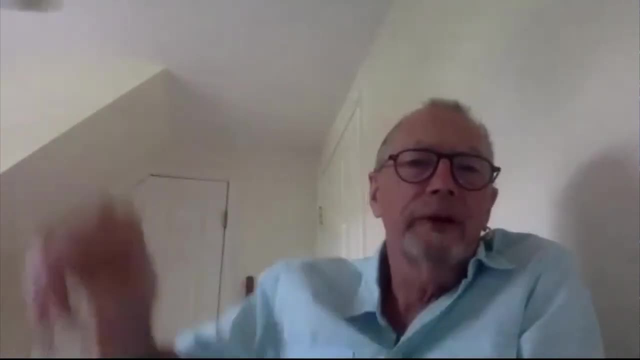 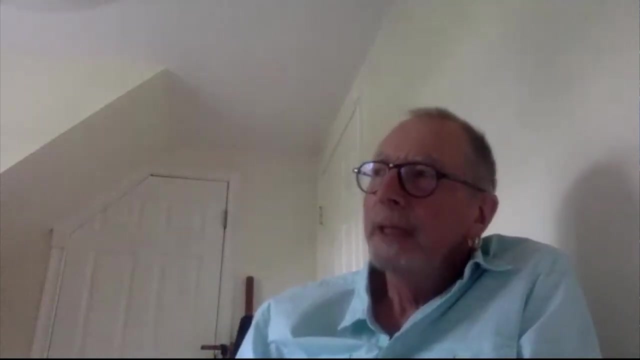 instead of saying that something is provable, you can just say: well, it's one of these numbers. where all those numbers are the, the numbers of theorems. so that's how you express things about provability. now, in girdle's proof you need a little bit more than that, because 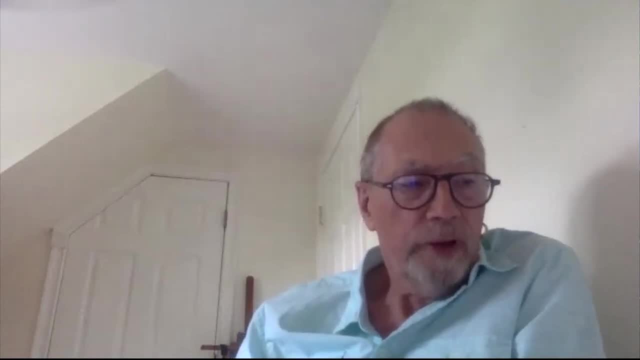 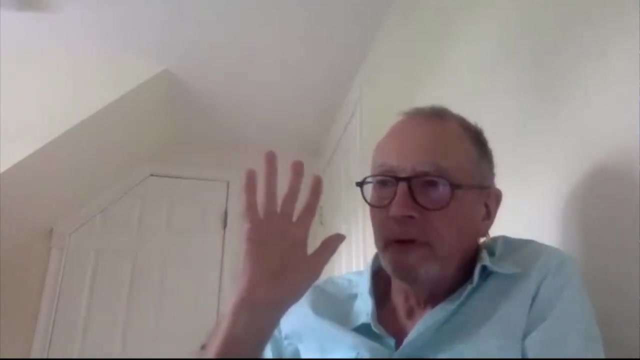 if you're going to code up this sentence which says: of itself, it's not provable, you need not only to be able to talk about provability, but you need some kind of reference, self-reference. so you need a sentence of the form: um n is not provable. remember, n is just a number, so the number of a theorem, um. you need something of. 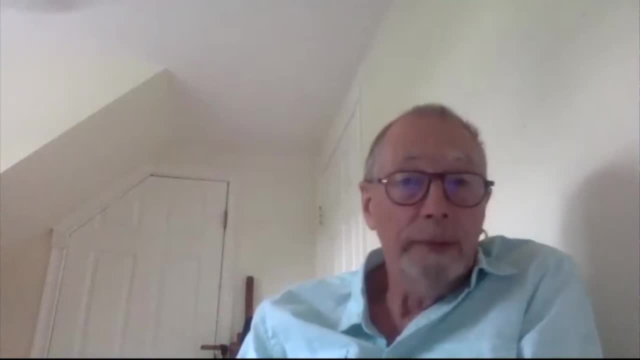 form n is not provable, so you need to have a number of a theorem. um, you need something of the form n is not provable, provable whose own code is N. then it's effectively self-referential. And perhaps the most ingenious aspect of Gödel's theorem is that you can do this. 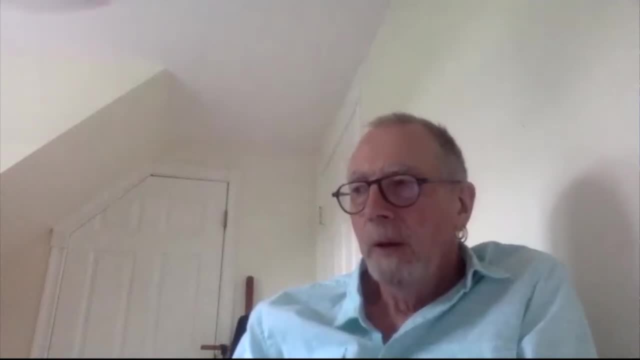 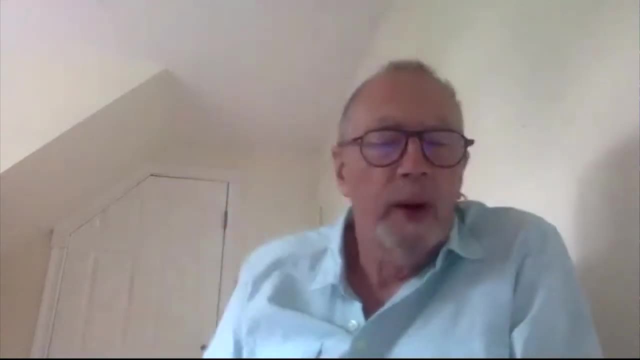 with a kind of fixed point construction. So this has been worked out. this part of the result in particular has been worked over at great length by many later generations, and now we know many more things about how you turn this fixed point trick than Gödel did. 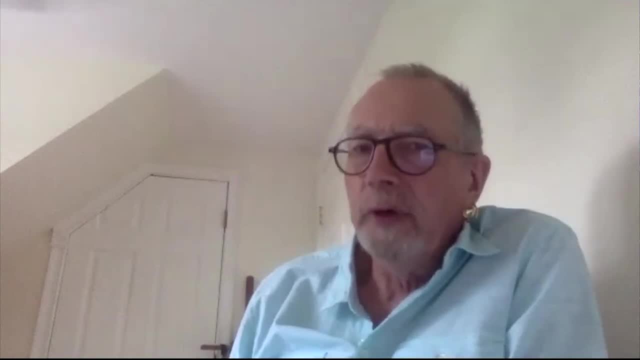 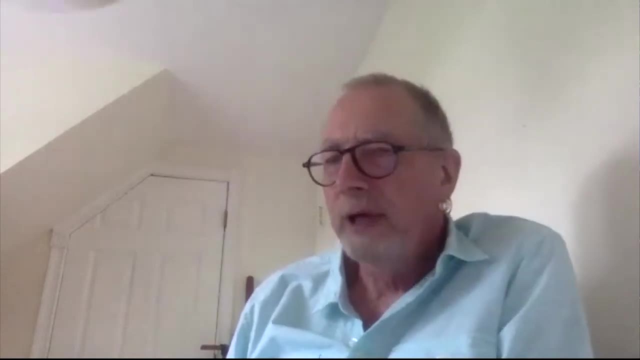 But showing that you could turn this fixed point trick, getting a number which had itself as its own code, was really, I think, the most clever thing of Gödel's proof. All right, so, given that you can then find this sentence and so intuitively it says: 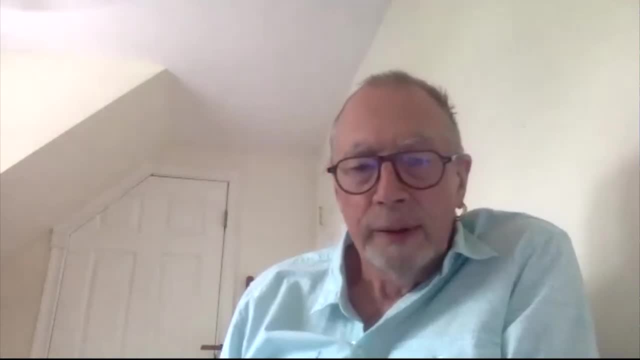 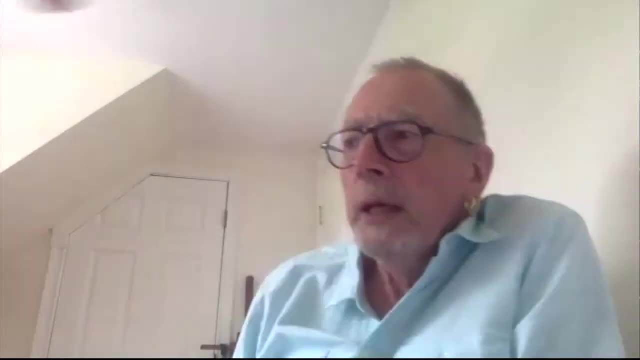 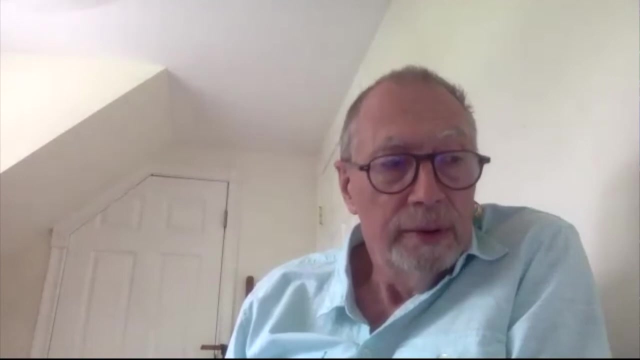 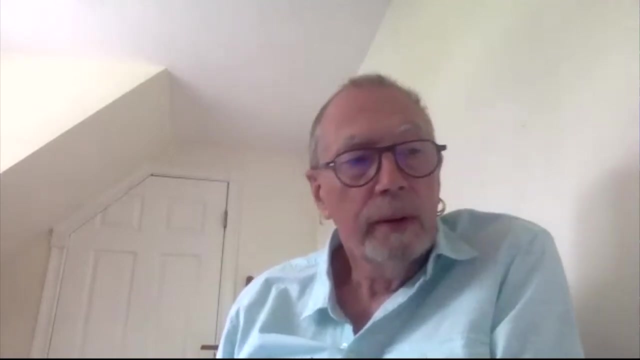 this sentence isn't proof, It's not provable, or it's a number, or it's a sentence, arithmetic, which says N is unprovable, which has itself code N. then you can try and push through the paradoxical argument and what you can show is that if the system is consistent, then you cannot. 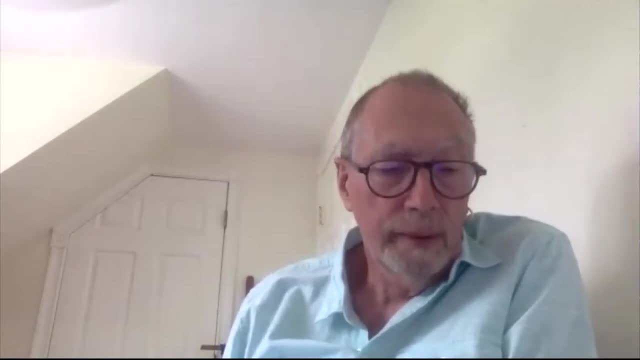 prove this sentence. Or, in other words, if you can prove it, the system's inconsistent. So, assuming the system's consistent, you cannot prove that sentence. But because you cannot prove it and what it's saying is true in the standard model, 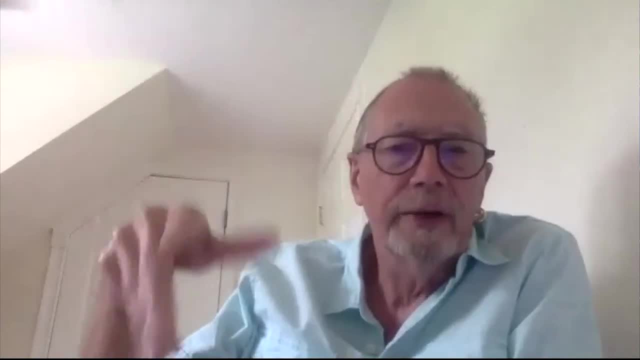 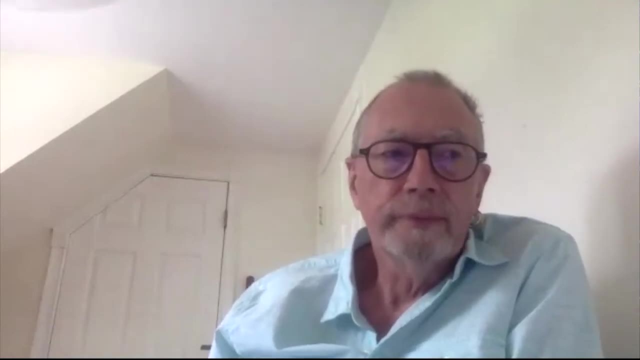 because you can't prove the system, so you do the decoding, et cetera, et cetera, and you can see that it's true in the standard model. this is itself a true sentence. So what Gödel actually showed was not simply. 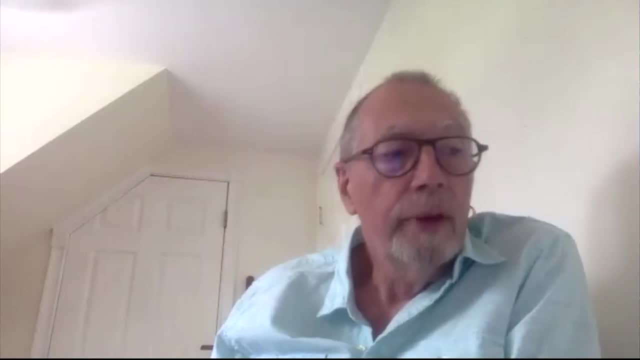 That the set of sentences true in the standard model is not axiomatized, well, not recursively enumerable. He actually showed something which is true in the standard model and it's not recursively enumerable, which is a lot stronger, Okay. So I mean, earlier on you said: well, how are you going to show this without setting? 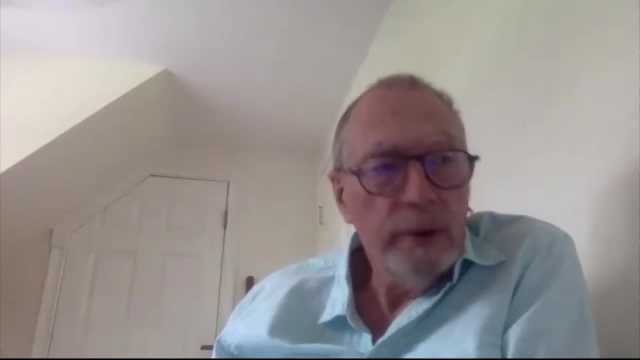 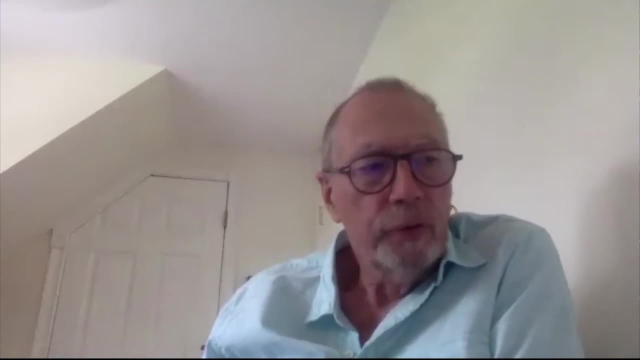 the truth or otherwise of some of these examples And you can do this, I mean, You might just have a very abstract proof that the set of true sentences in the standard model is not recursively enumerable. That will be completely sort of non-constructive proof. 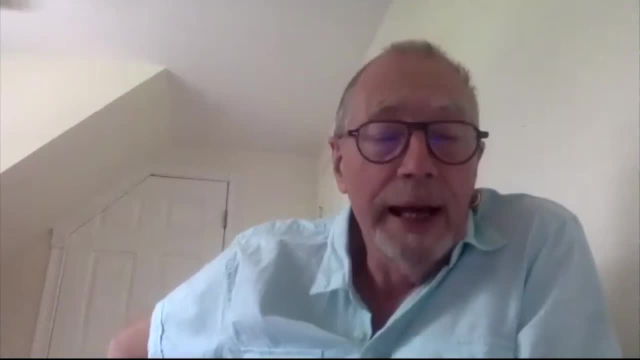 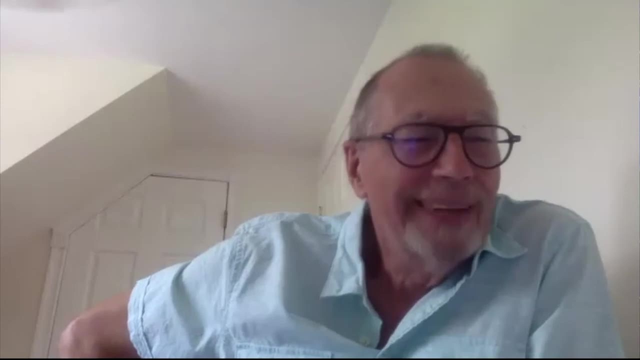 But Gödel achieved more than that, because he showed: given an axiom system, you can actually pin down one of these bloody things and it doesn't look terribly interesting for mathematicians. okay, Who cares about a sentence which says it's not proof? 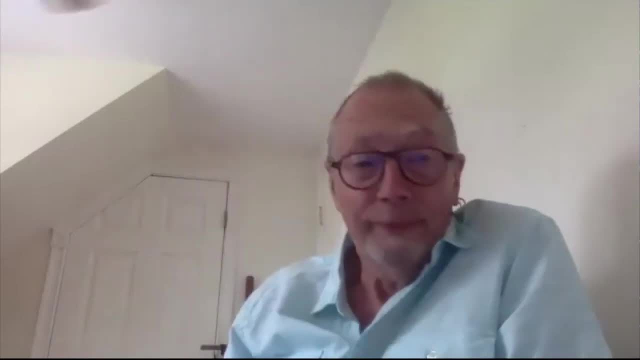 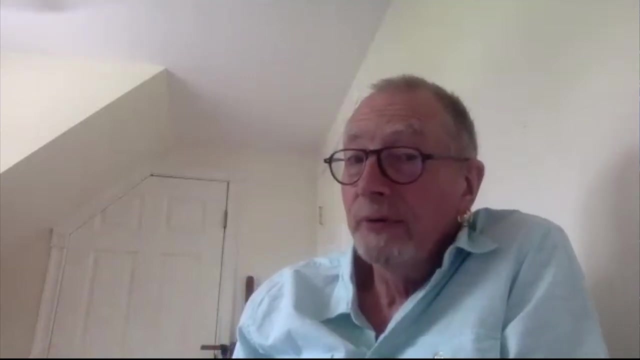 You know this is a party game But kind of interestingly, in the 70s and 80s mathematicians came up with some genuine mathematical, contentful, mathematical issues which can't be proved in first-order arithmetic. All these standard axiomatizations are a large fragment thereof. 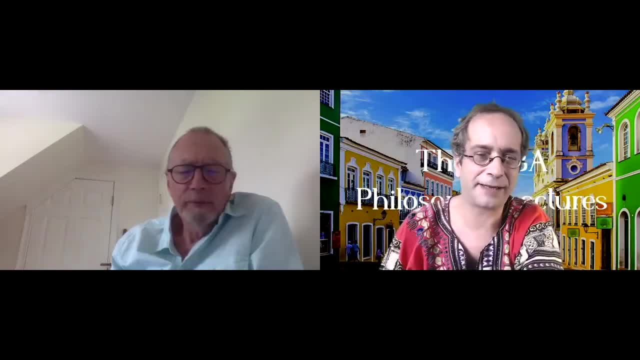 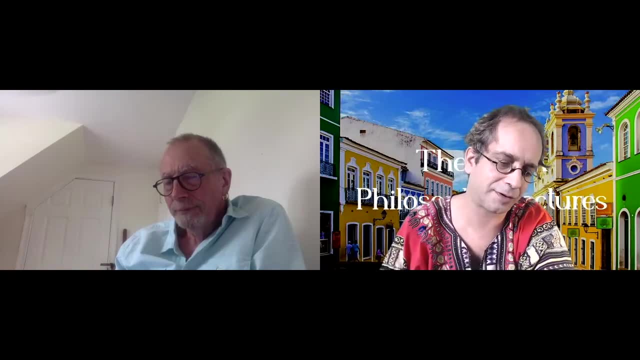 We could go into those if you'd like. but Yeah Well, in fact I was about to ask you to come Comment on the form of these Gödel sentences and if there are, of course, some interesting sentences of this kind. 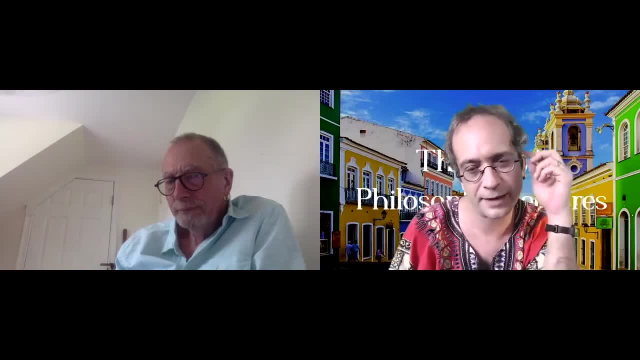 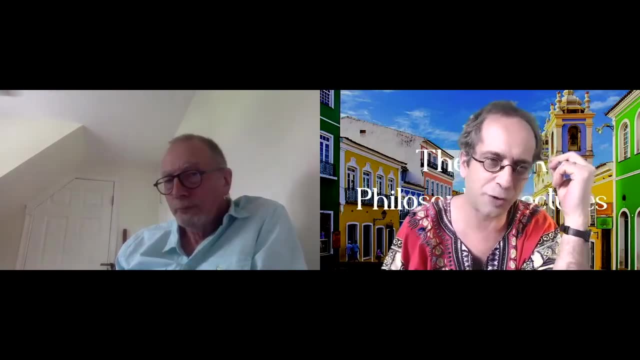 So yeah, I think I would like to get into that. What is the general form of these Gödel sentences? I mean, I suppose of course they must contain a universal quantifier, But what more, I mean, can we know, judging by the form, if a sentence is undecidable? 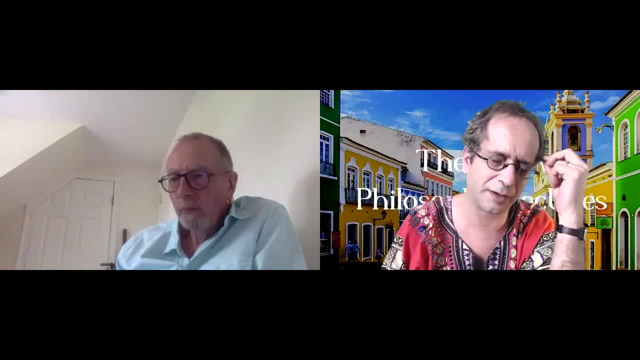 No, Yeah. so all the sentences without quantifiers are going to be provable. All the true ones are going to be provable. So it's only when you get the quantifiers involved, get these sort of Hilbertian ideal elements, that the situation can arise. 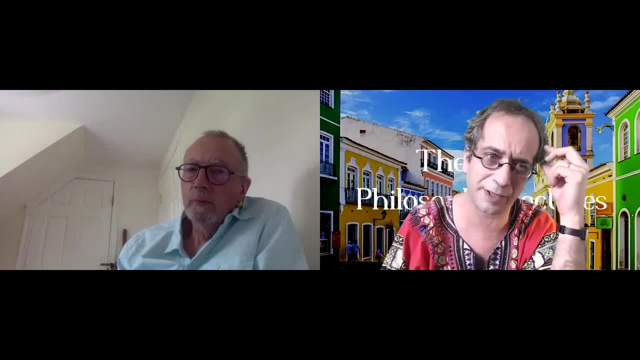 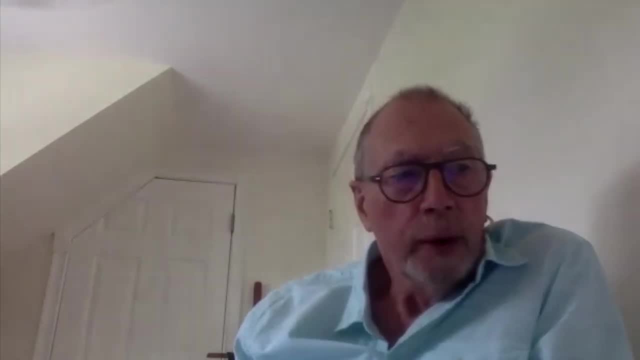 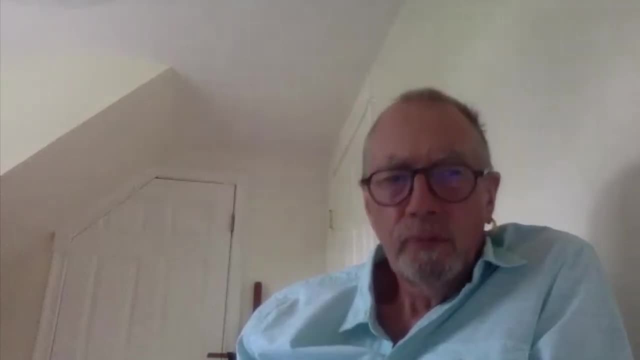 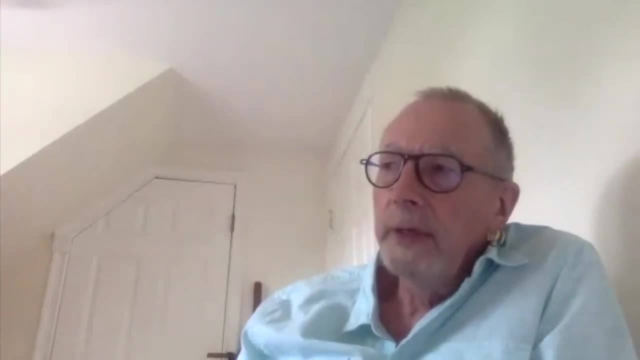 Yeah, Yeah, But the undesirable senses are not all of this strange form. So I mentioned that in the 70s and 80s some mathematicians established some quite interesting problems in mathematics whose truth can't be established in standard expertisations of arithmetic. 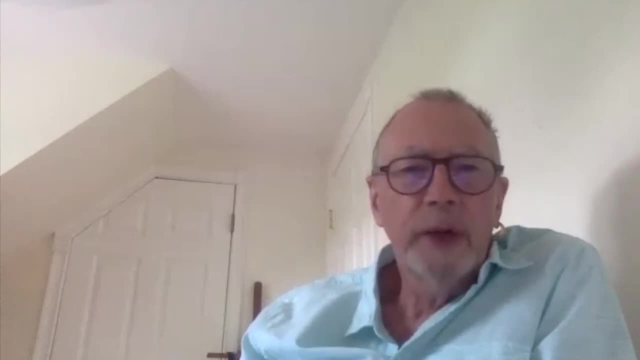 And it's reaching the limits of my knowledge here, But I seem to remember that one of these is the pigeonhole principle, which says something like this: If you've only got a finite number of pigeonholes, and you've got an infinite number of pigeons, 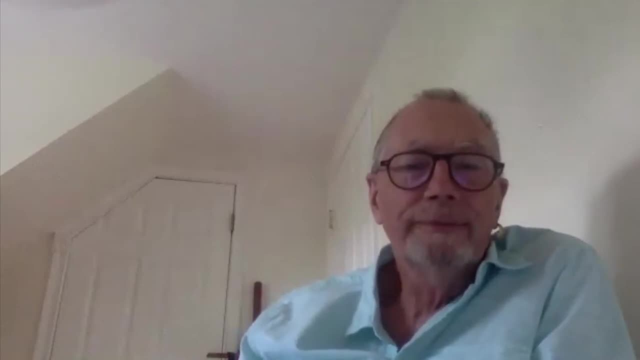 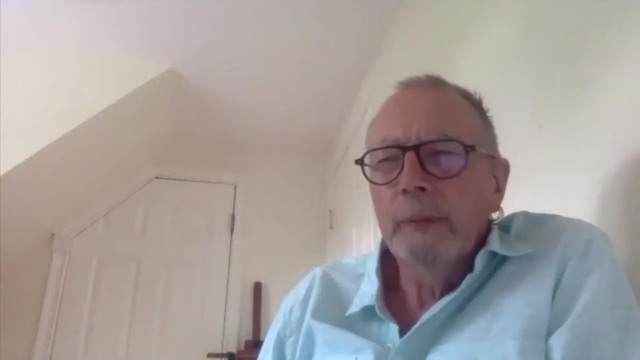 then you've got to put at least two pigeons in one pigeonhole. This is the pigeonhole principle. You can express this in terms of numbers And I think that what some mathematicians showed- maybe Geoff Paris, but, as I say, 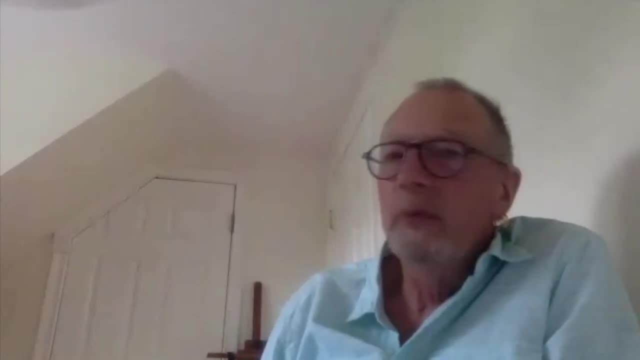 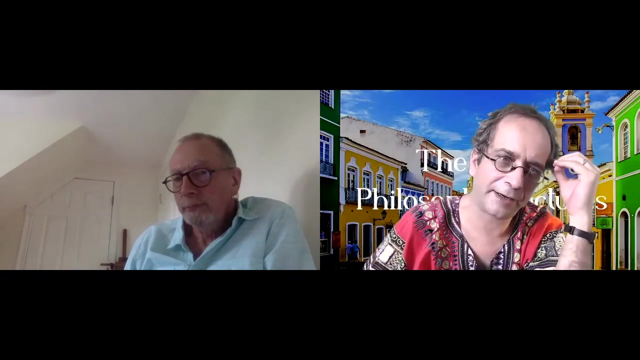 I'm reaching the limits. of my memory here was that you can't prove the pigeonhole principle in standard expertisations of arithmetic And some Diophantine equation or something to do with Diophantine equations too, if I remember well right. 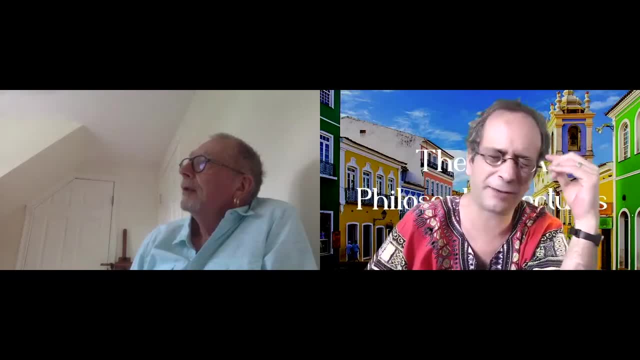 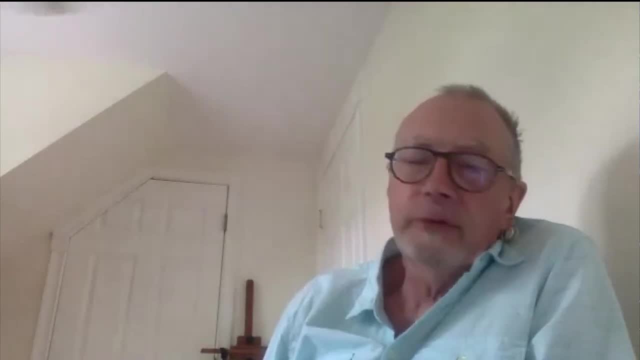 Yes, that's right. Something to the effect that there is no general solution to Diophantine equations, or something like that. Yeah, So this is a very famous problem enunciated by Hill Hilbert in the year 1900.. So it's called Hilbert's 10th problem. 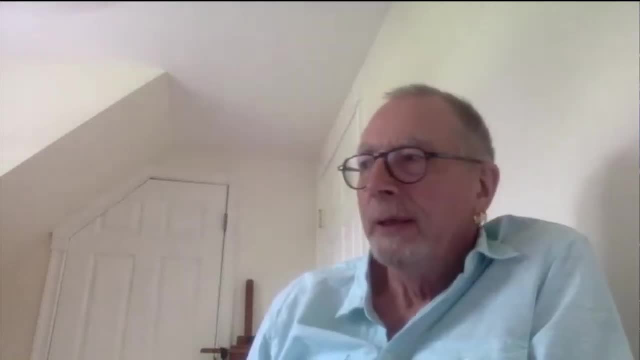 If you've got a Diophantine equation, which just means a polynomial equation with integer coefficients. like you know, 5x cubed plus 3x squared, plus x plus 2 equals 0. And integer solutions too, Yeah. 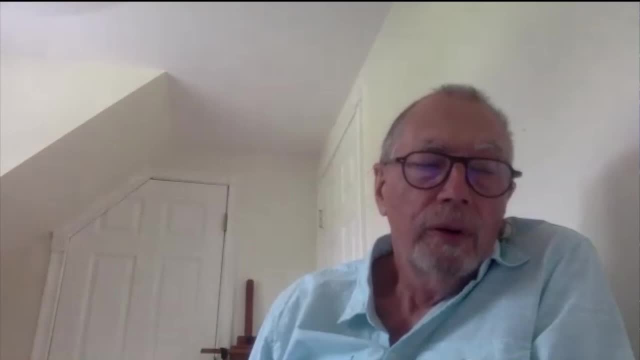 Right. Can you always solve equations of that form? Yeah, You can't, And you can prove that you cannot. You can. That was a famous unsolved problem. It was proved when that result was proved- in the 70s I think. 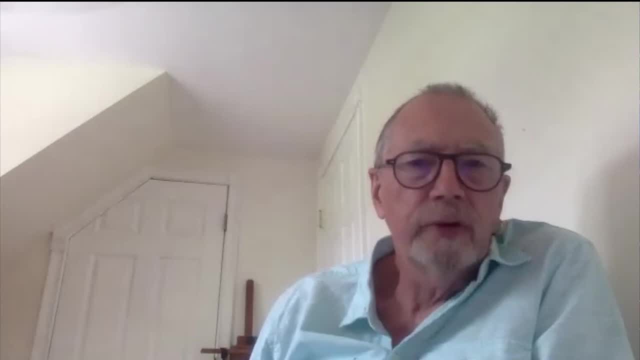 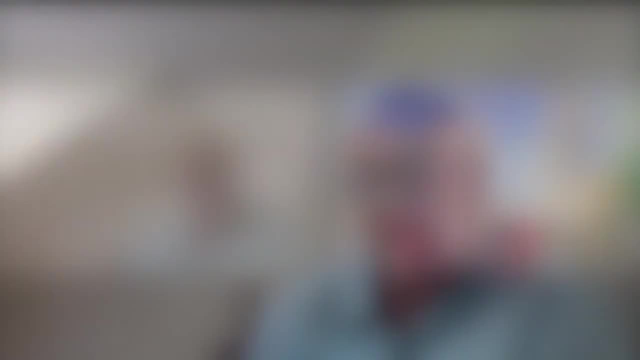 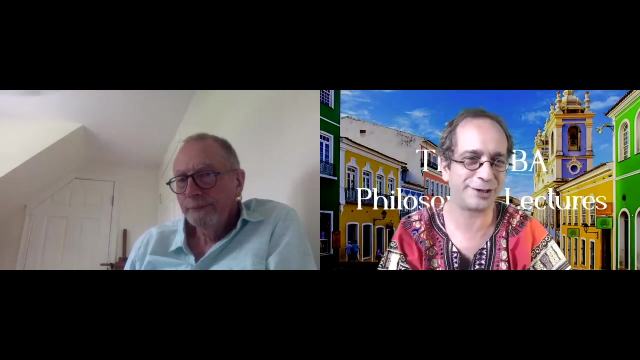 maybe late 60s by Matjasevic, building on the work of a number of other logicians, But he's usually credited with this result. Hermann Weyl said that Gödel's result was draining his enthusiasm for his research in mathematics. 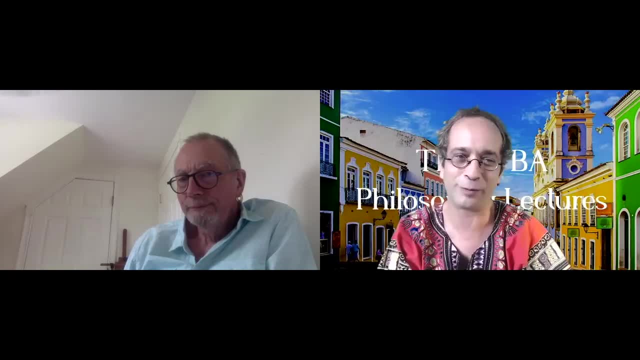 because he could no longer know whether the problem he was working was of a Gödel kind or not. But going back to the form of Gödel's sentences, So let's call Gödel's Gödel's sentences, all the infinitely many sentences. 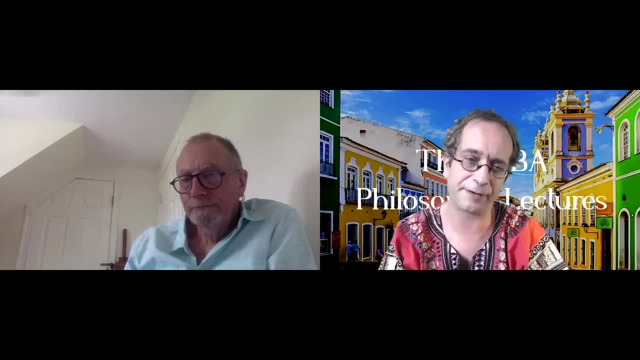 that you can build in various different codings that you can come up with, Is undecidability co-extensive with Gödel's sentences? I mean, suppose that you know that a sentence in arithmetics is undecidable. Do you thereby come to know that there is a Gödel number? 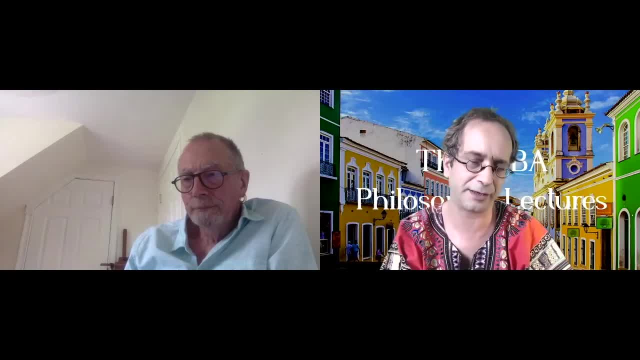 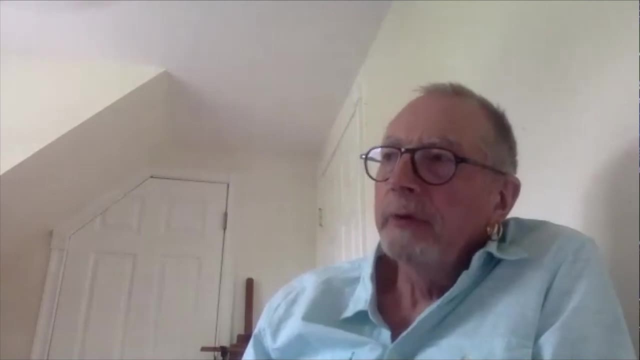 or some kind of coding which produces that undecidability? Or are there other ways in which non-Gödelian ways in which a sentence could be undecidable? Sure, Look, I mean, any sentence is going to have a code. 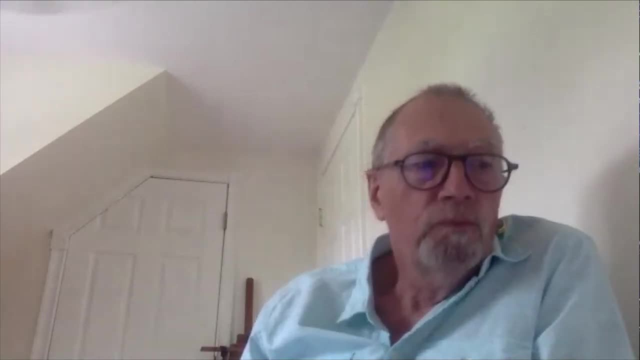 because you can cut up every sentence. So every unprovable sentence is going to have a code. Every provable sentence is going to have a code, But that doesn't mean that every undecidable sentence is going to look like a Gödel sentence. 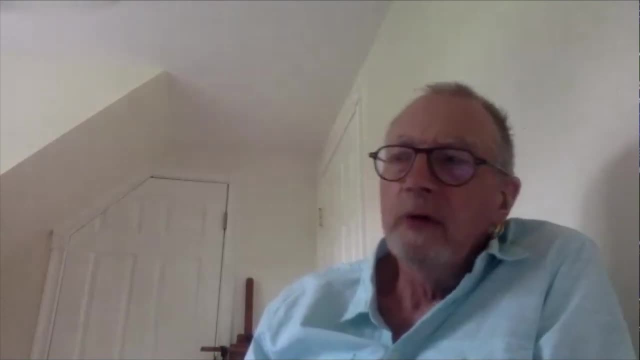 in that it applies self-reference. So you know this pigeonhole principle. if I've got it right, and that's unprovable in, say, piano arithmetics, standard axiomatization arithmetics, that doesn't look anything like a Gödel sentence. 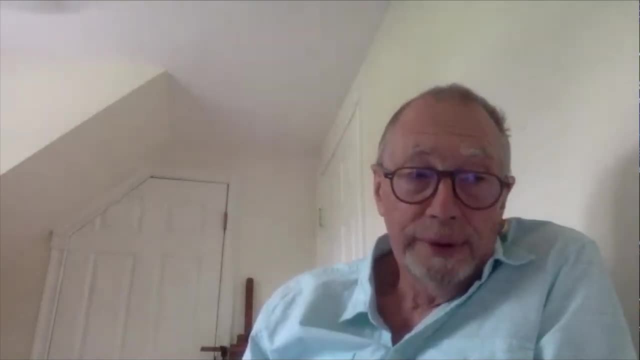 Actually, you know, once you get to set theory, matters become much more complex and interesting, because set theory is incomplete as well. It contains arithmetic. so you know it's going to be incomplete, but it's going to have more interesting, more interesting incompletenesses than just arithmetic. 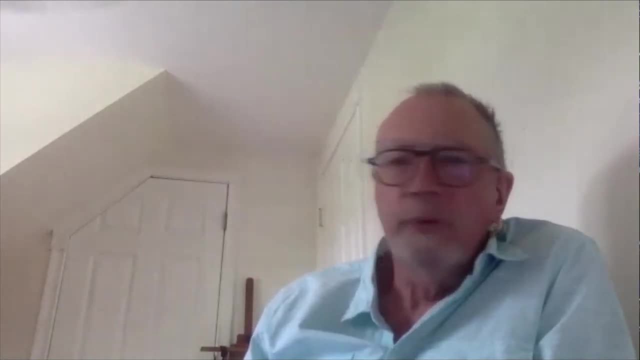 And there are many famous problems of set theory which are insoluble in standard set theory. So once I'd like to continue my hypothesis. So once you move from arithmetic to set theory, things become much more complex But in some sense more interesting.